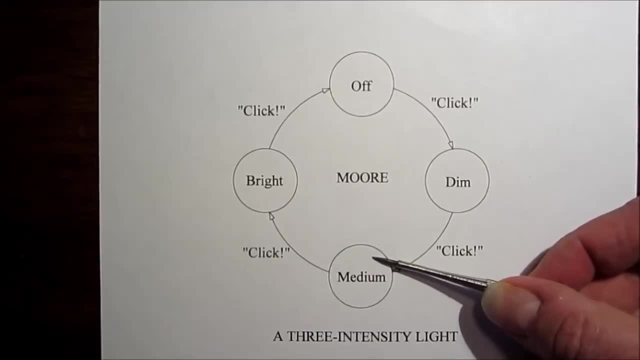 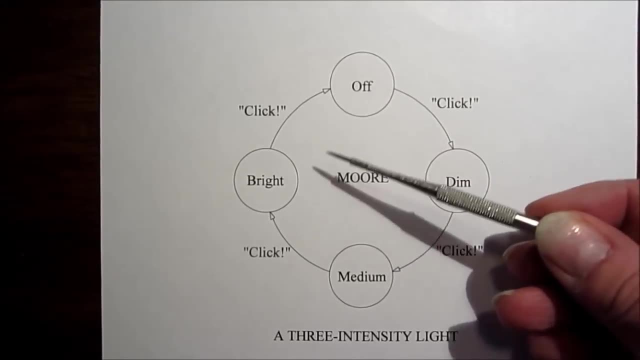 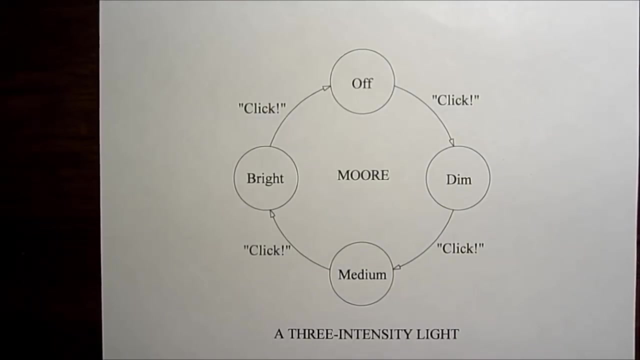 to dim when we click the switch. Then we click the switch again and it goes to medium, Then it goes to high and then it goes back off. So we have four states here. Now in a Mohr machine we would represent the output or the status or the state of the outputs inside. 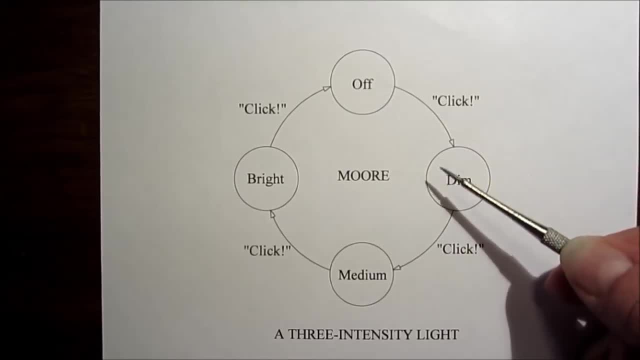 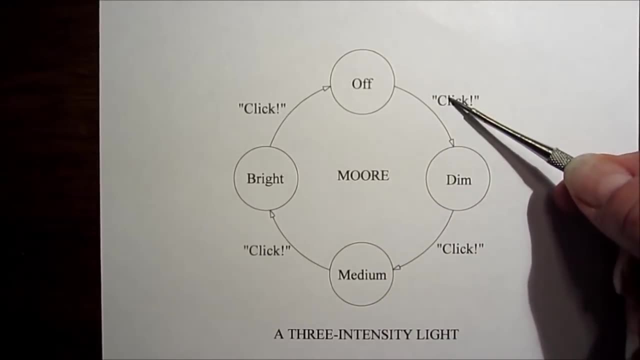 the state bubble. So here we have off, we have dim, we have medium brightness and we have most bright. And these are the conditions that cause it to change state from one state to another. Some action Here, it's a click of the switch. Now in a Mealy machine we don't. 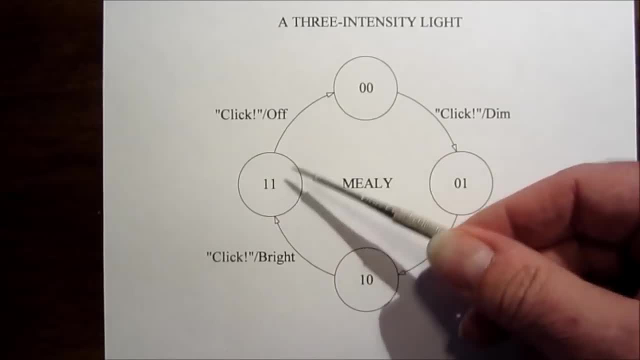 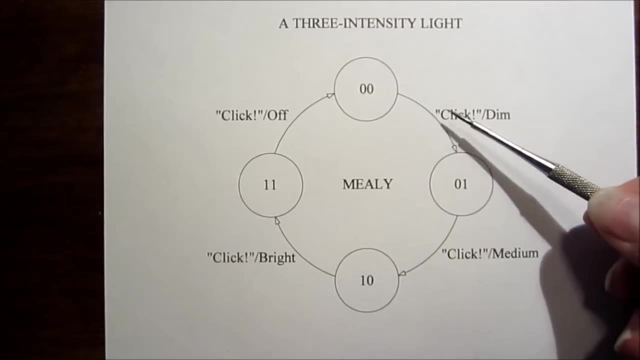 show the status of the output inside the state bubble. We show it outside the state bubble, As a matter of fact, we show it in combination with the conditions that caused the state machine to change states, In other words, the transition. So here we have a click and we 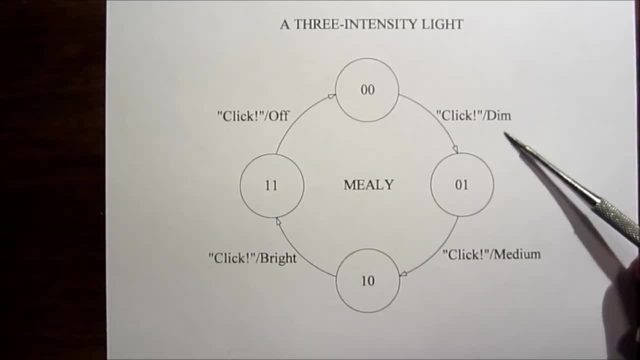 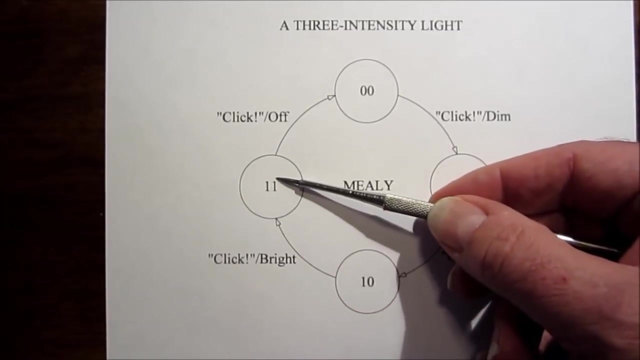 output a dim, We go into a dim condition. Now this is just kind of an abstract placeholder, if you will. Now we have another click and we output a medium condition From this state. we have a click and we go to a bright condition. Now we're in this state. Then we have another. 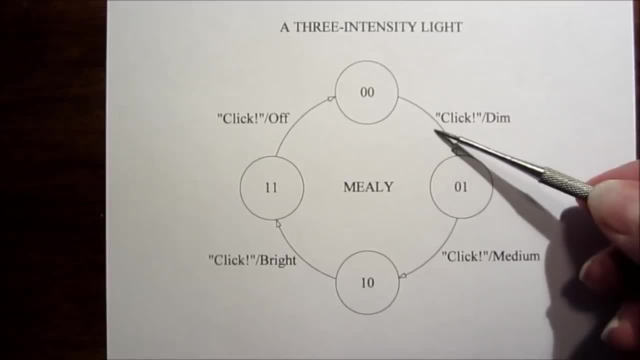 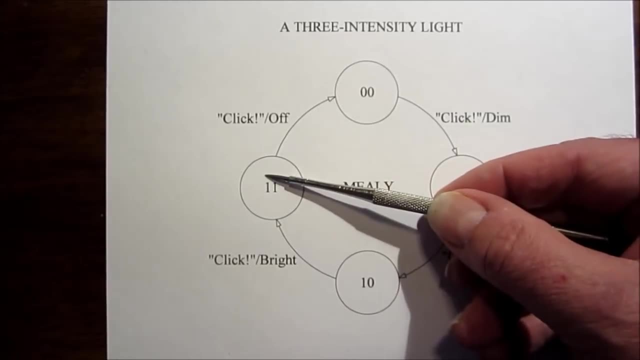 click and we turn it off. So we notice. the difference between the two is that the Mohr machine said off: dim, medium and bright here. Here we just have the state indicators, which can also be in the Mohr machine, But we have 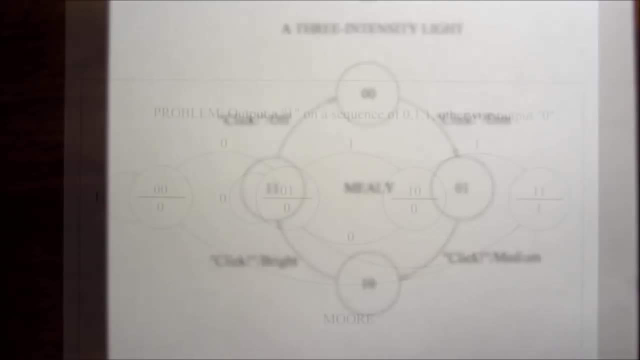 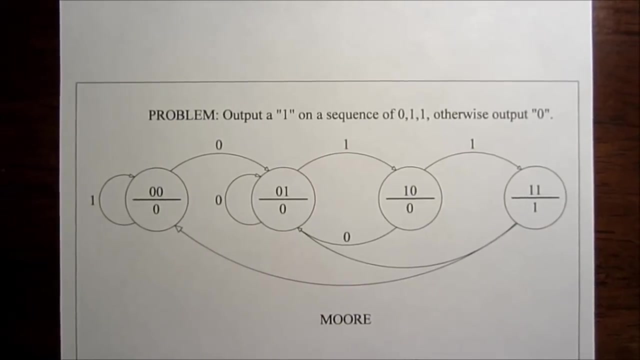 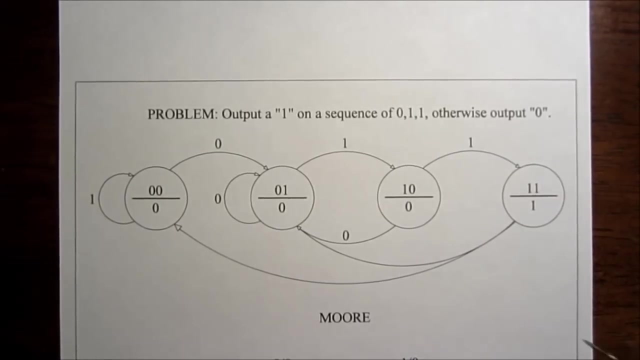 the main thing is the output is here in the transition. Now let's say we want to build a state machine that can observe an incoming stream of bits and tell us when a 011 sequence has occurred. This is the way the Mohr machine would work. Now, Mohr machine, we have the state. 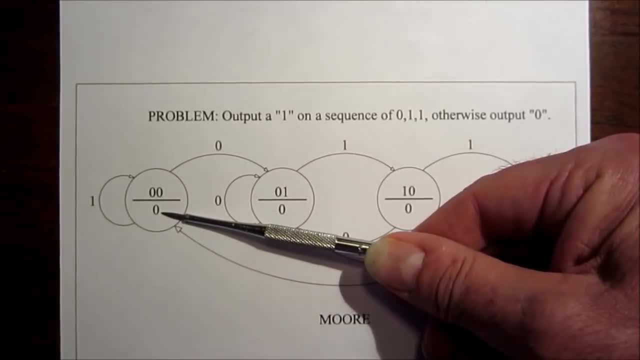 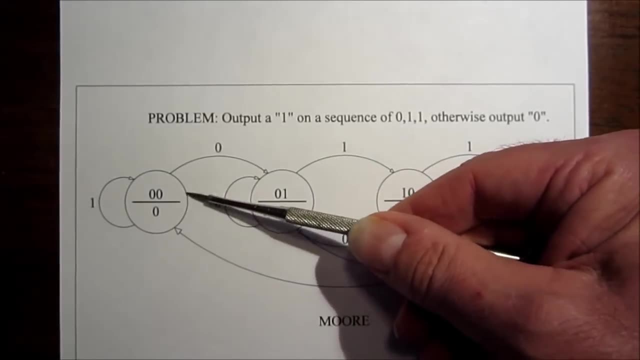 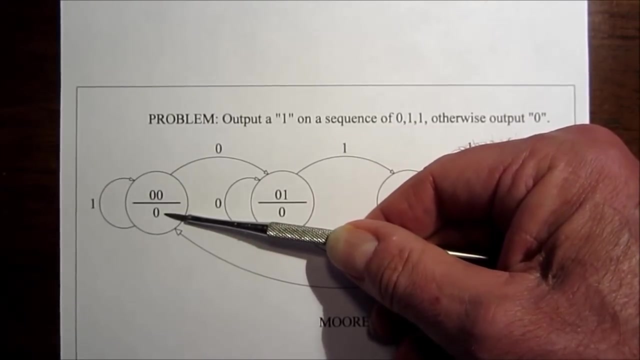 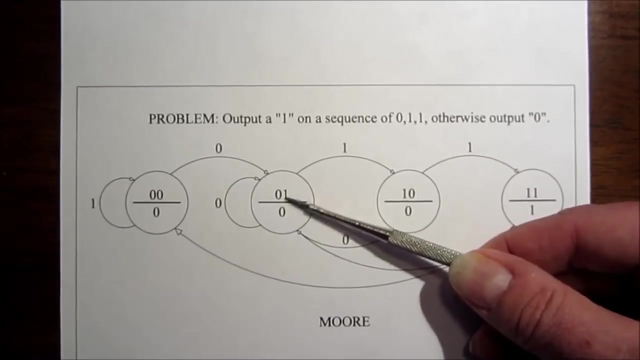 number here, And then we have the output condition listed with the state number. So it's inside the state bubble. So here we are, in state 0. And we're outputting a 0, which means we have not seen a sequence of 011 yet. If a 0 occurs, we're going to transfer over to this state. Well, first of all, if we're 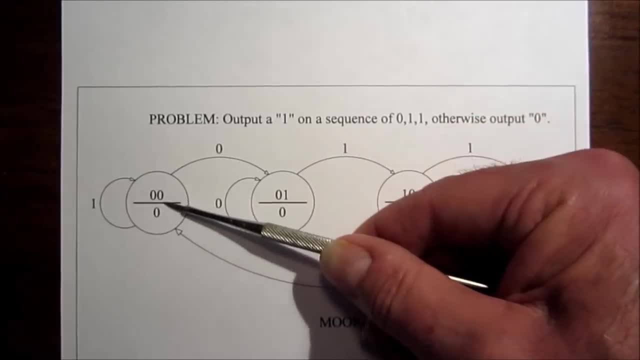 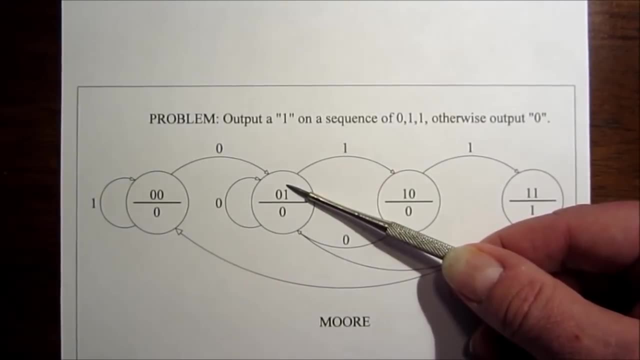 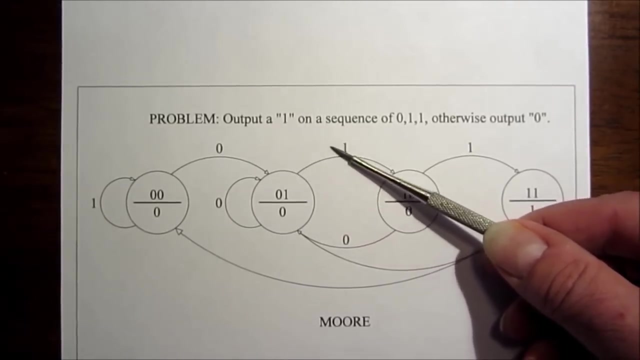 in the 0 state and a 1 occurs. we haven't started yet, So we just go straight back to the 1.. If we get a 0, which is a candidate for the first bit in that sequence, we will transfer over to this state 0,1. But we still output 0.. Now let's say we have a 1.. Well, we're well. 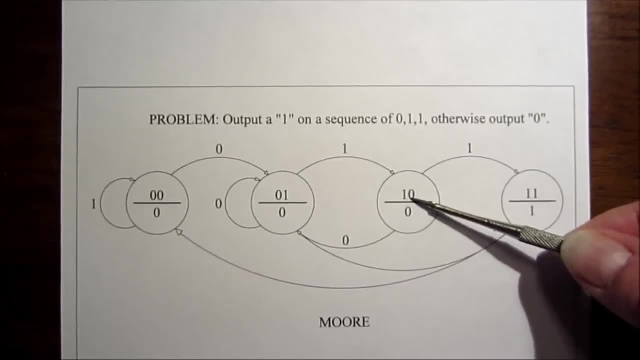 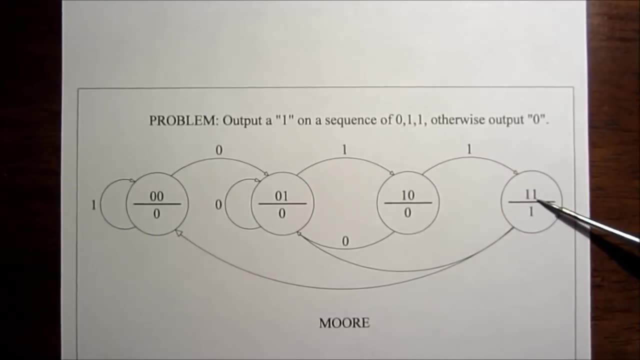 on our way now to our sequence. So we transfer over to this state, But we still don't have our full sequence, so we're outputting a 0.. If we get our second 1, we have completed our sequence. We transfer to this state and we output a 1.. Then we automatically have a 0. 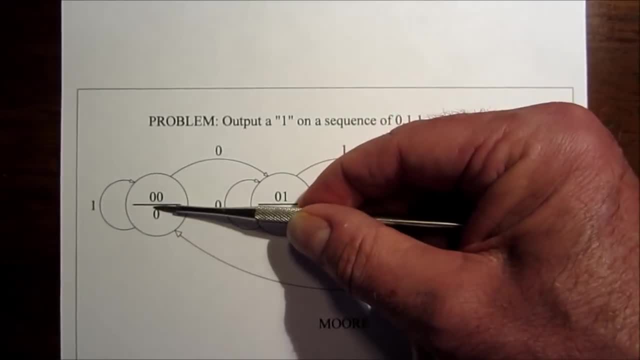 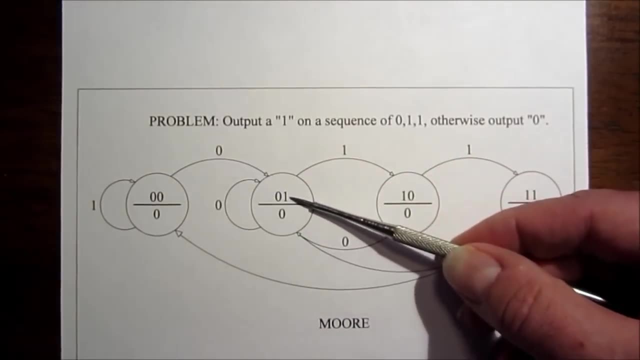 Now the problem is that when we transfer the last sequence to a state that we just showed, we automatically go back to this beginning state and we wait here again. Now, if we've gotten a 0,, 1, we're waiting for the last 1, but we don't get it. we get a 0,, we go back to this state. 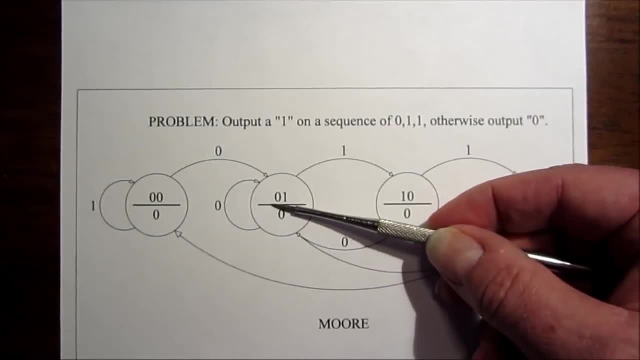 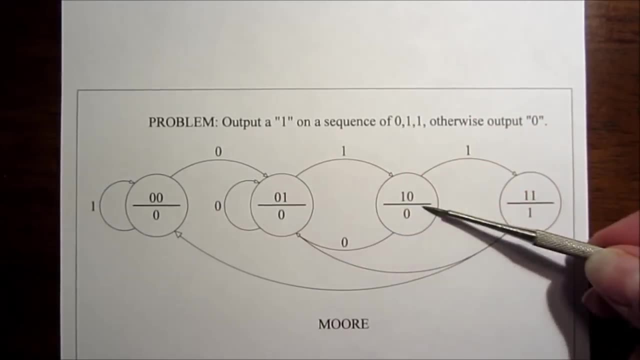 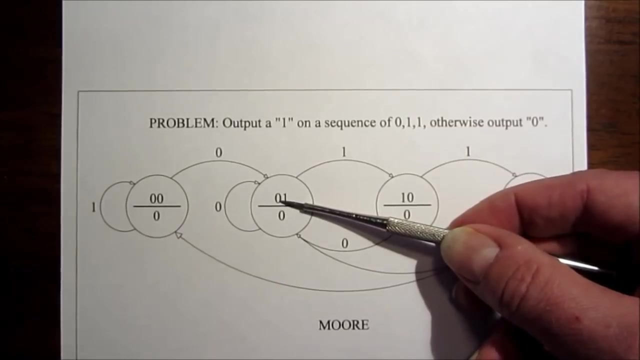 because we just got a 0, that really could be the first 0 in the next sequence. So, depending on where we are in this state machine, for instance, if we go from we have a 0 and then instead of a 1 we get another 0, again we go back. 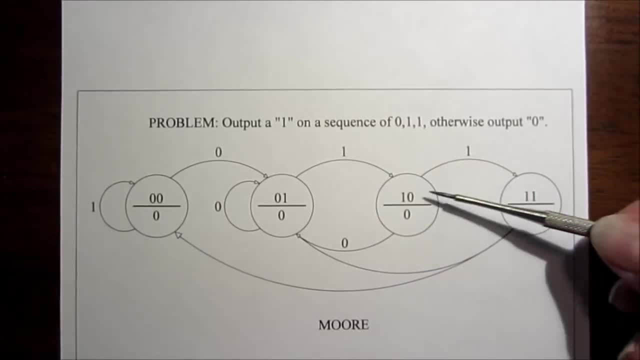 to this state here waiting, But it's not until we actually get the full sequence that we go back to the original 0, 0 state. The important thing about the Moore machine is that it has its outputs here inside the state bubbles. 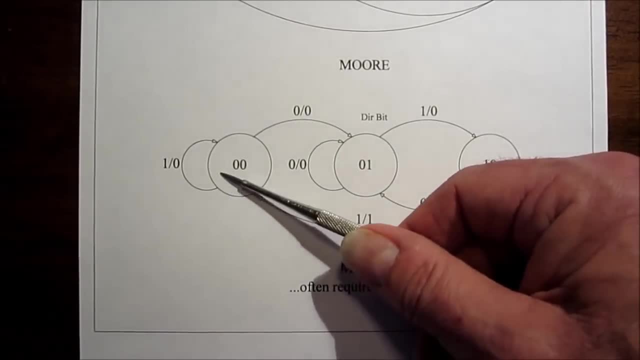 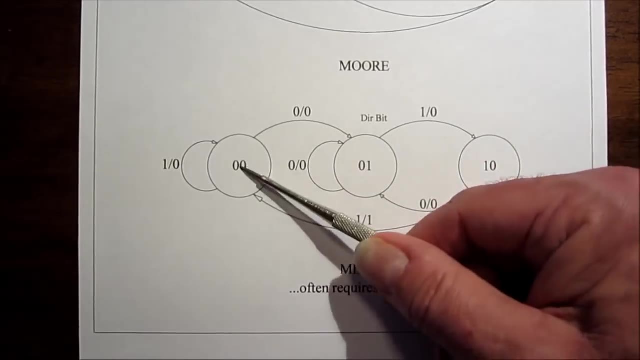 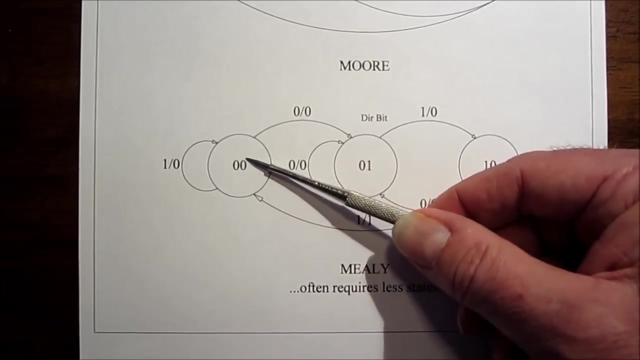 Now, as we said, the Mealy machine has its transition and its output both listed in the transition arrow, So inside the state bubbles themselves we just have the state number. So in this case we start off here in state 0, 0. 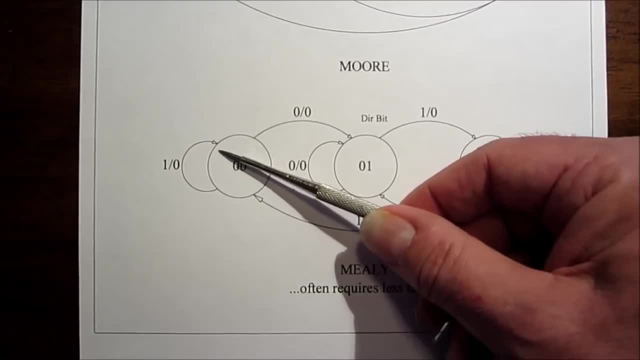 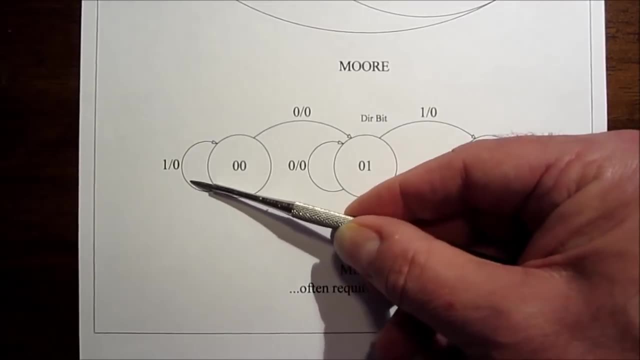 we're looking for a 0, 1, 1 sequence. If we get a 1, it certainly doesn't start us off. So we're right back here again, still waiting, And we're saying: well, we've got a 1 and we're outputting a 0. 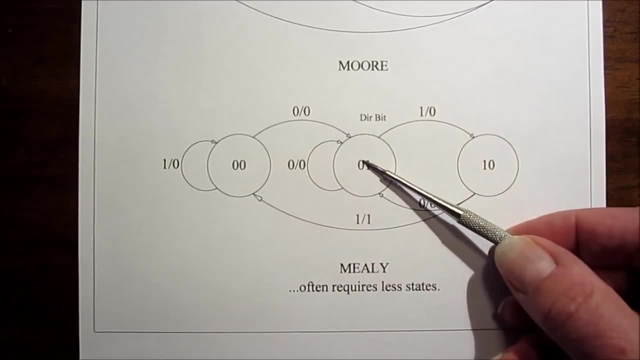 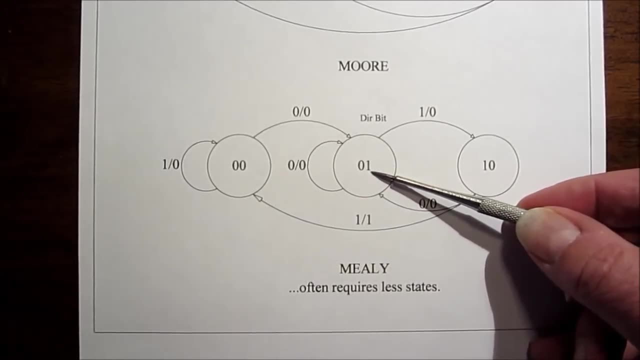 meaning we don't have our sequence yet, But if we get a 0, we're going to transfer over to this state. Well, so far, we look quite a bit like that previous Moore, because now if we get a 0 instead of a 1, we stay here. 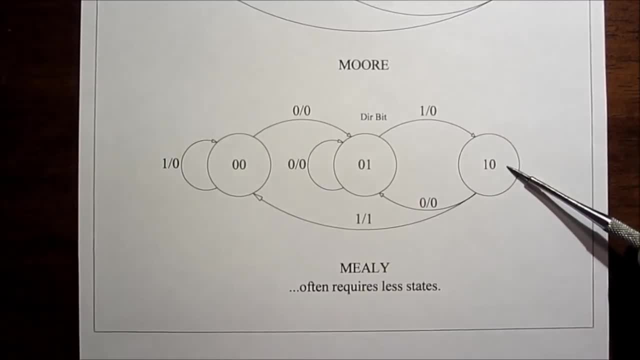 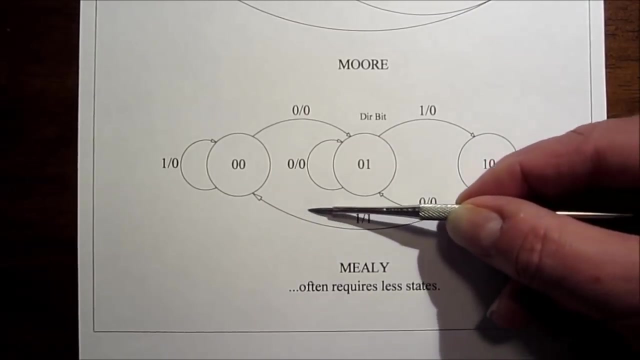 But if we get a second one, we go here. Now, if you recall, the Moore machine went on to one more state over here for another one. But here we've gotten a 0 and a 1.. We're waiting here Our third one. we go straight back. 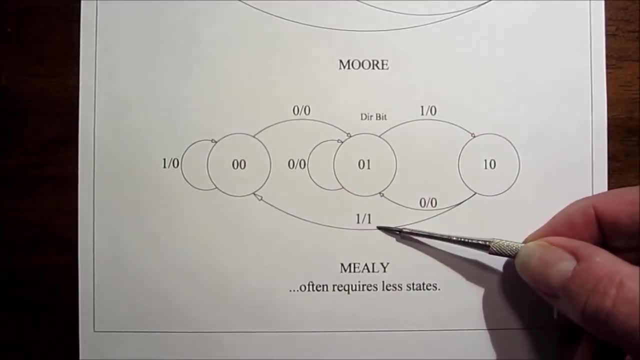 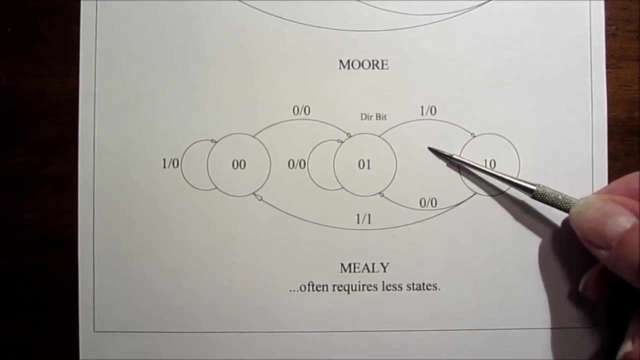 to the original position and we output our bit to indicate that we have found a 0,, 1, 1 sequence. So the bottom line is: we've done the same job with one less state. So the Mealy machine often requires less states to accomplish the same thing. 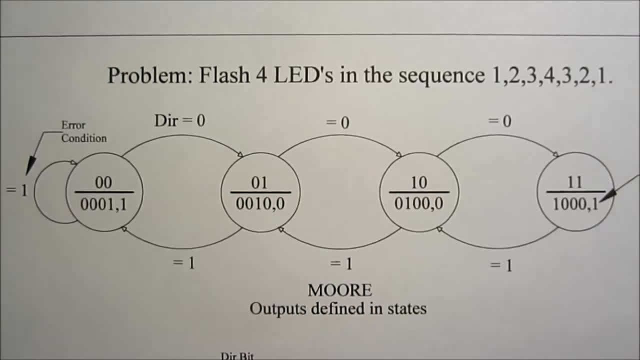 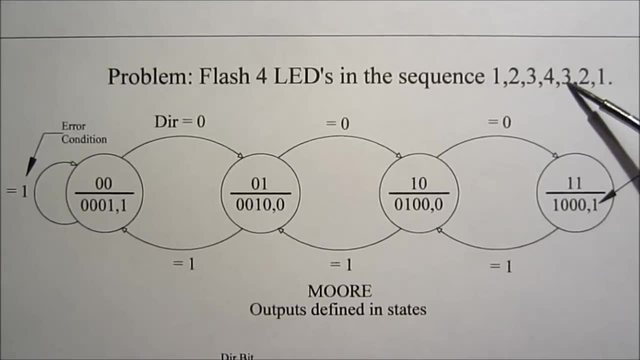 Okay, let's look at another example of how the Mealy and the Moore machines might handle the same problem. Here, what we want to do is we want to sequence four LEDs in a sequence of 1, 2, 3, 4, 3, 2, 1, so that's what we'll want. the 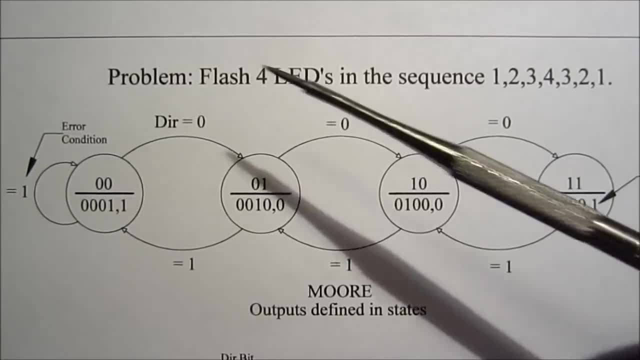 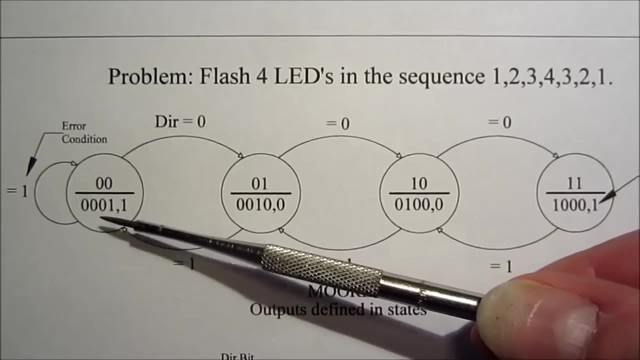 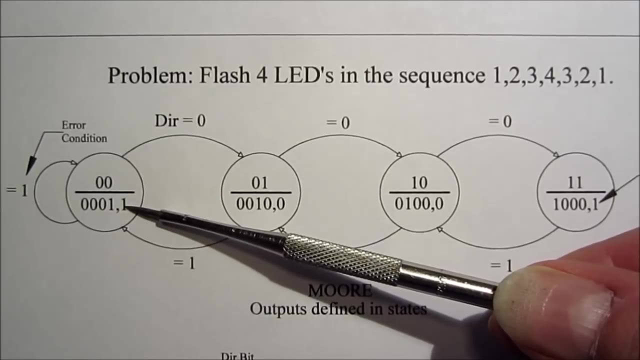 state machine to do, And in a Moore configuration, we start off here with state 0 and of course, we have our output shown on the inside of the state here. Here's the LED that we have turned on, and this bit right here is going to be a toggle bit We'll get back to. 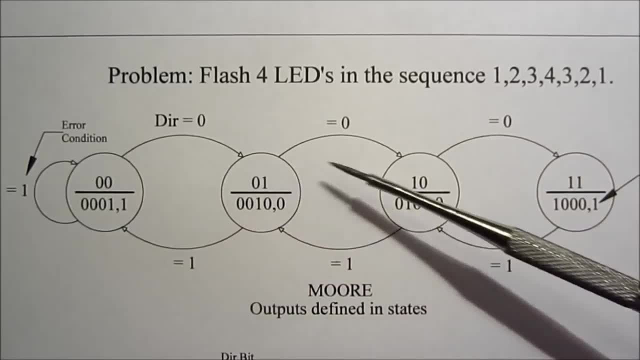 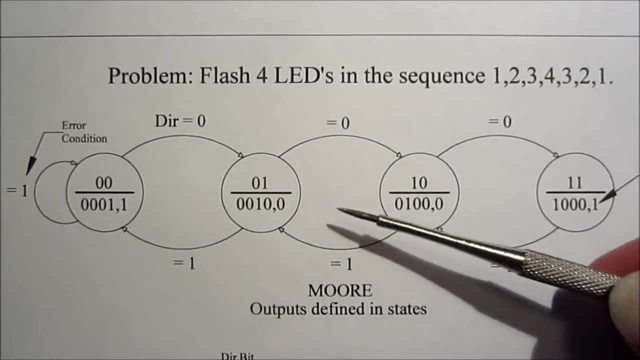 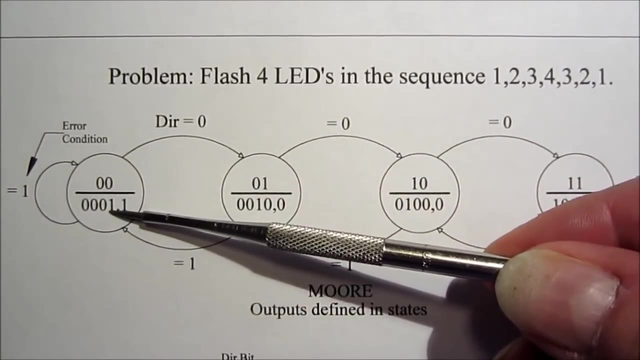 that in a minute. So right, Right here we have our state number, we have our output, which- this is the LED and this is a control bit that goes to a toggle register or a toggle flip-flop. Here we have our error condition if we ever end up here in this state with the wrong direction. 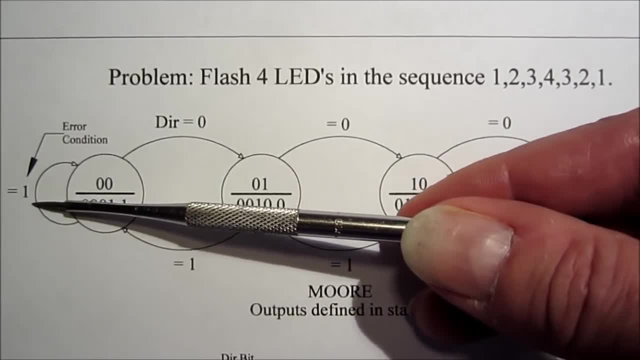 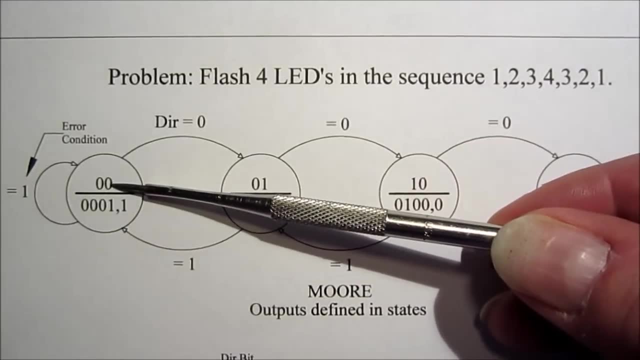 bit set, we can fix that. In other words, if we have a direction bit of one set at the zero, zero state, that doesn't make sense. We should have a zero set. So we just loop back here. and what happens when we loop back? we set this one here and 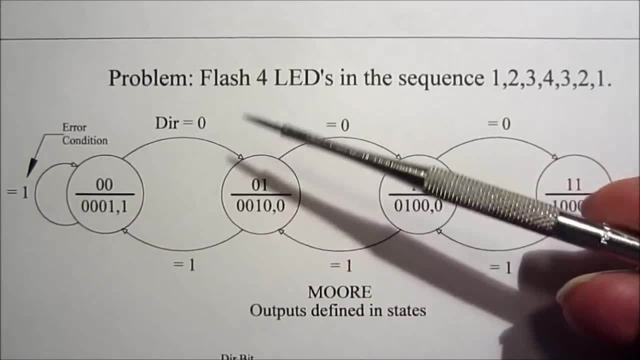 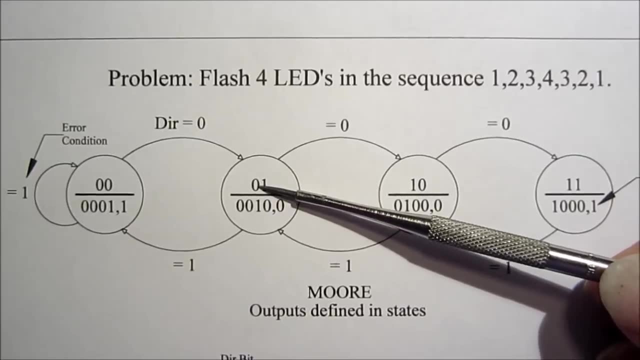 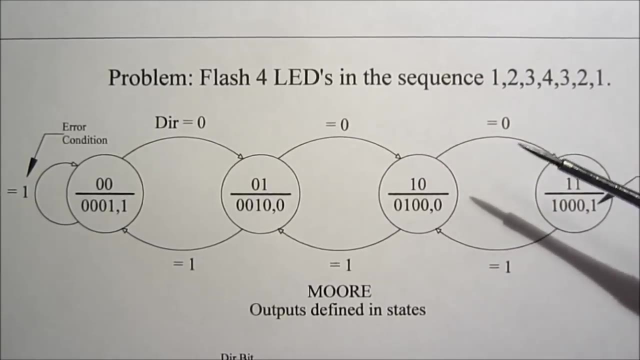 we toggle from a one to a zero. So if we start off here and we move to the first state when the clock clocks the chip and then we again move this way each time. now looking at this direction, bit for guidance. So we know that in this direction, 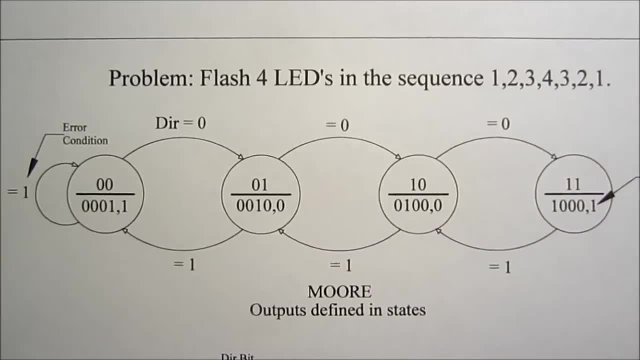 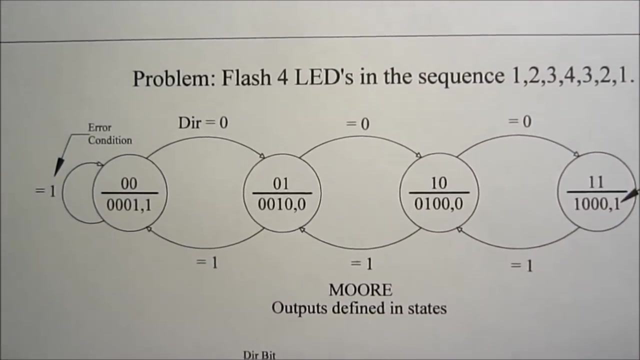 The direction. The direction bit is going to be zero and in this direction it's going to be one. So when we get down to this state with the last LED here, we toggle the toggle bit, We toggle the toggle register. So it says toggle the direction bit. 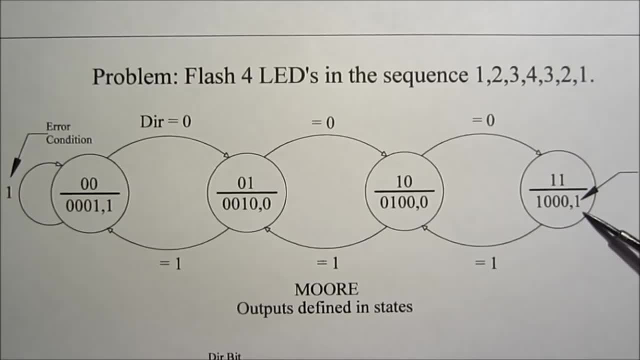 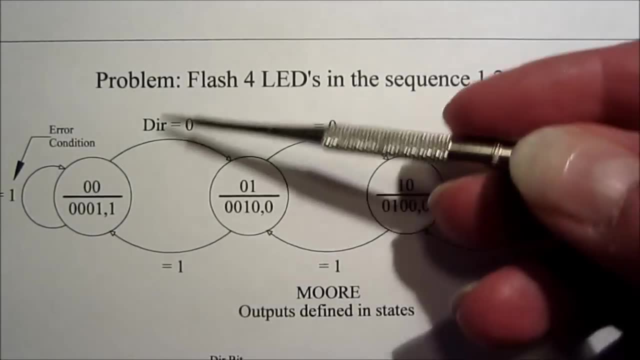 So you'll notice that in this machine, right here at this end of the line and over here at that end of the line, we toggle the direction And that's how we manage which direction we're going to change, which state we're going. 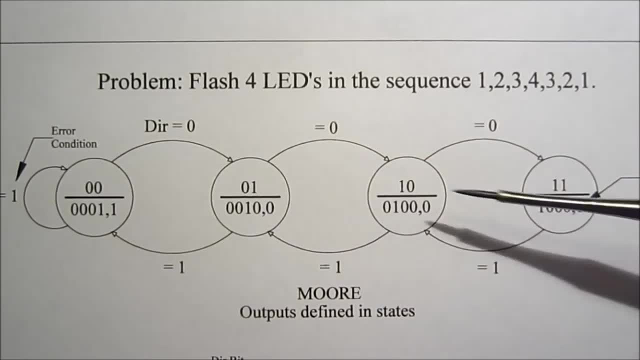 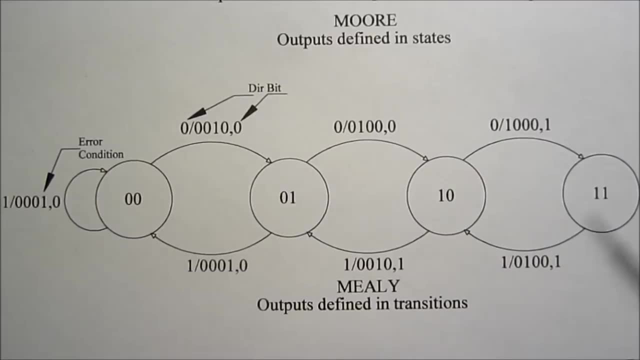 to go to next, because, especially in these two states, you could move in this direction, or you could move in this direction. Now let's look at the way a Mealy machine might handle the same scenario. We start off with state zero, zero, and likewise we have a direction bit. 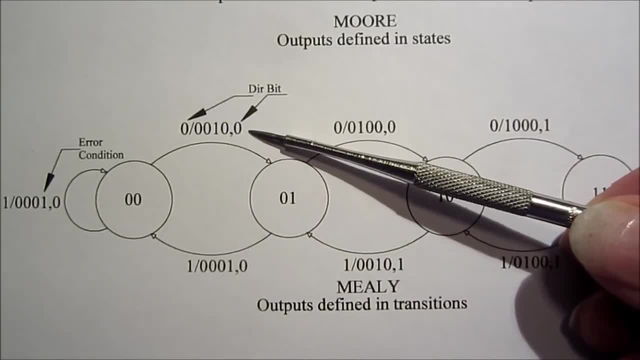 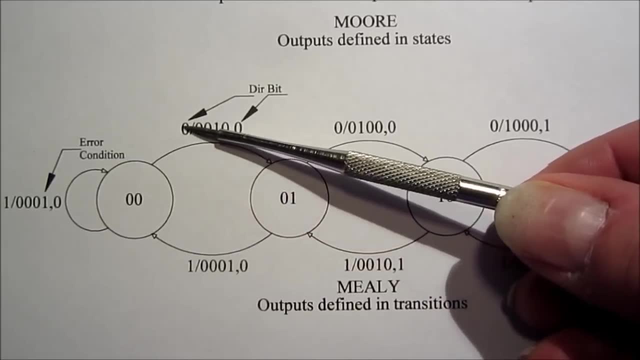 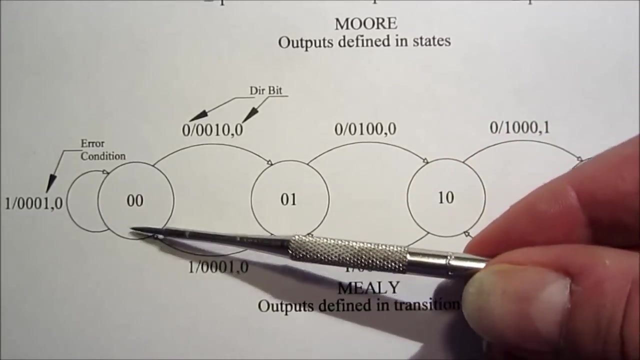 We're looking at the direction bit right here, but we're also setting the direction bit. So in this state right here, We make a decision: If the direction bit is zero, we're going to move in this direction. If the direction bit is one, it's an error and we correct that. 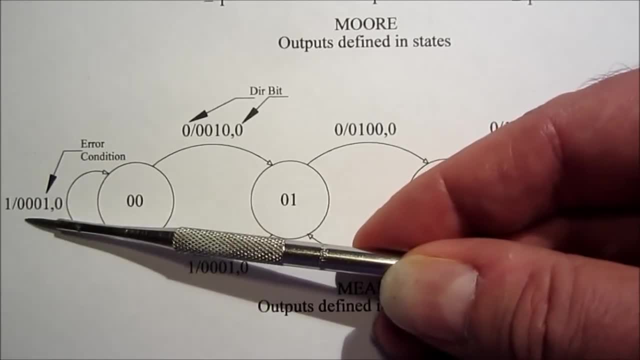 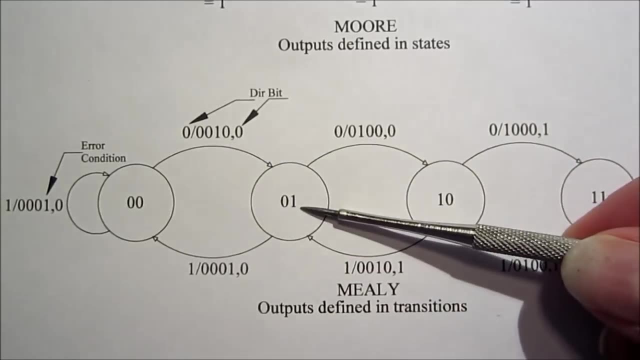 If the direction bit is a one, while we're in the zero zero state, we set it to a zero. Now we've got everything set up to where we can move in the right direction. So we move to this state and then we set the proper LED here. 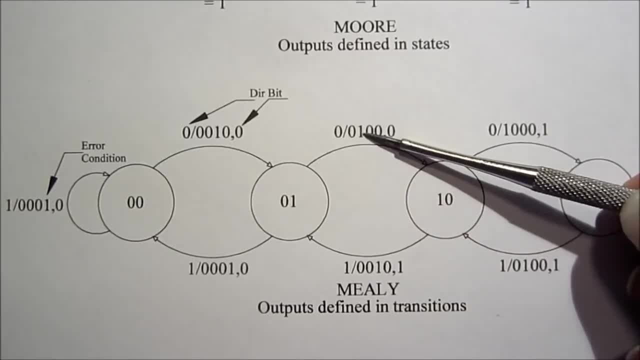 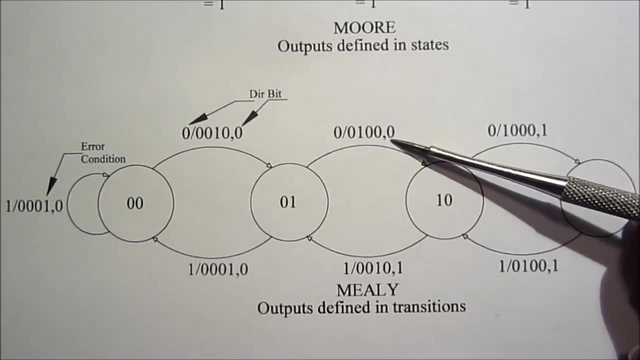 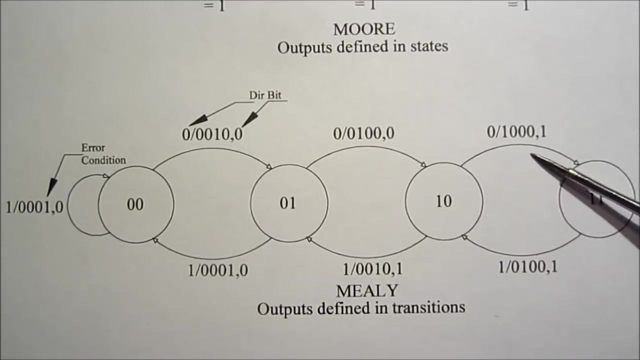 Remember, in a Mealy machine all of our transitions indicate Both of our inputs and our outputs. Now we're also setting a direction bit of zero here, which is continues on in this direction. But when we get to this state and we move in this direction, we set the direction bit. 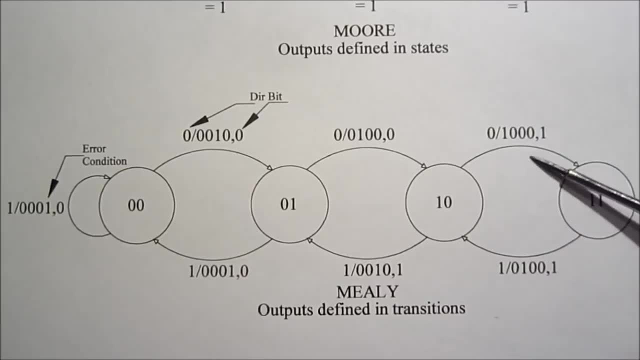 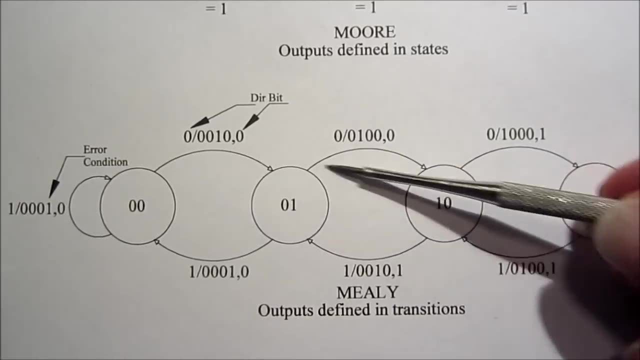 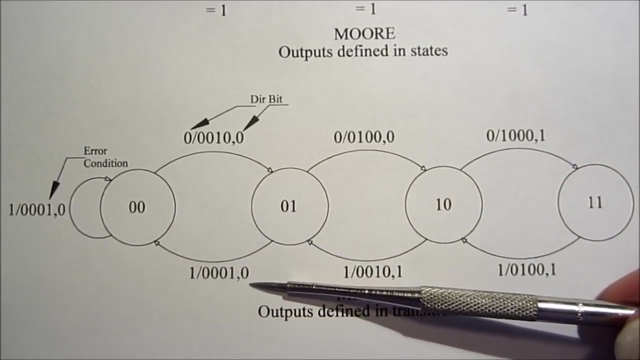 of one. So now we've prepared to move back in this direction. So now, here we see a direction bit of one in this direction, just like we were seeing an input of a direction bit of zero moving in this direction. And when we get back here, we reverse the process and we output a direction bit of zero. 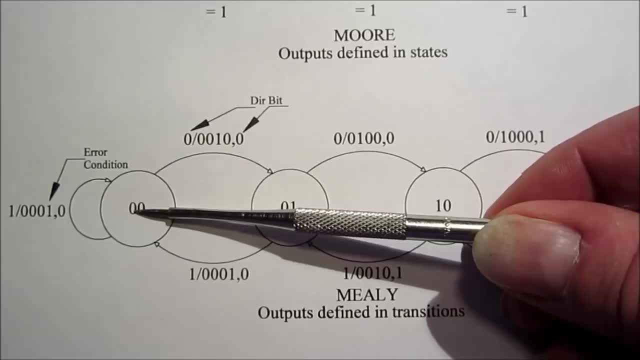 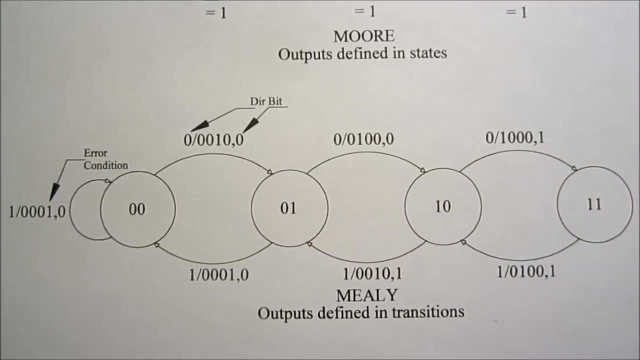 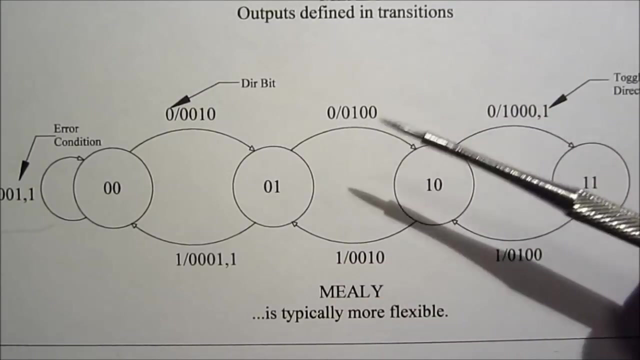 right before we transition into this state, or as we transition into this state, simultaneously really. And now, on the next clock, we have our direction bit set correctly. Now, you will recall in the last example that we gave, which was the Mealy machine above. 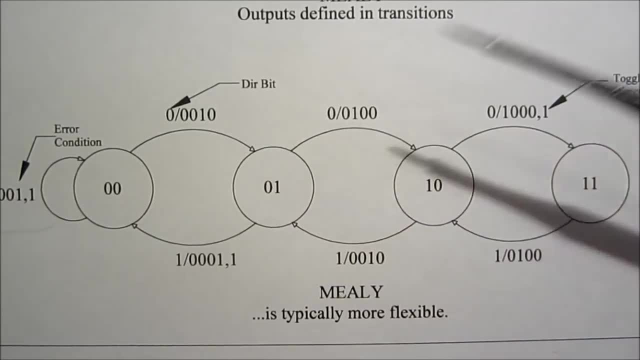 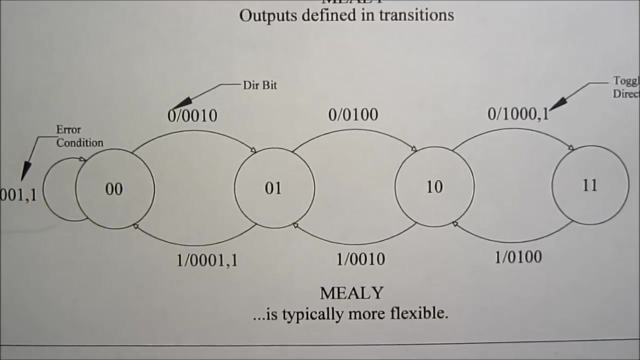 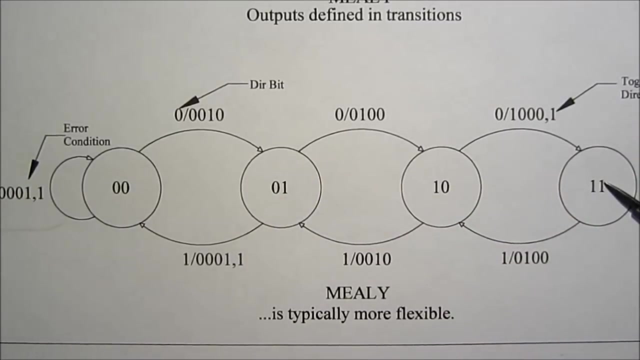 this one That every time we changed states in these transitions, our output included a specific direction bit. So we were specifically defining the direction bit at each transition, Whereas in the Moore machine that we looked at at first, what the Moore machine would do is it would toggle the direction bit through a toggle flip flop at each end. 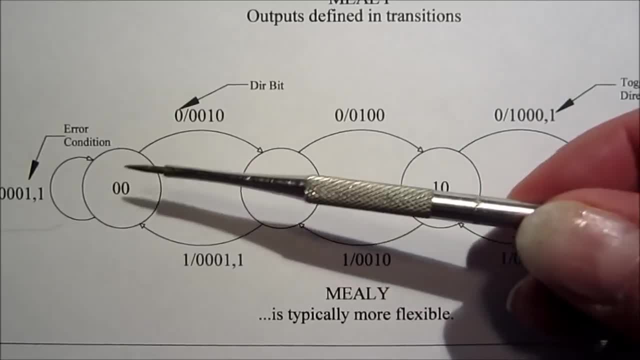 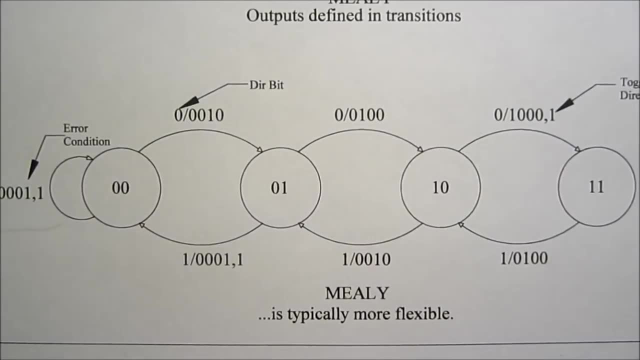 At this end. It would toggle from a zero to a one, and then it would get back here and it would toggle and it would go from a one to a zero. Well, here we have a Mealy machine that does exactly that, So it can emulate the behavior of that Moore machine. 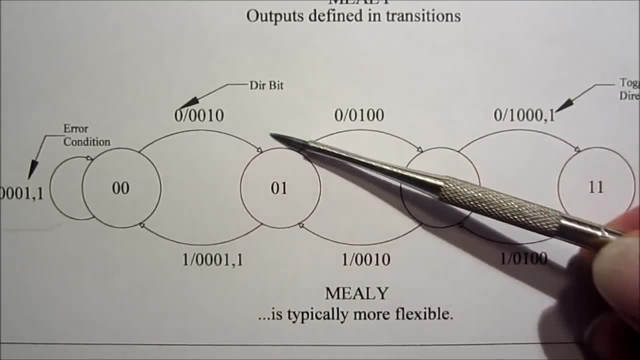 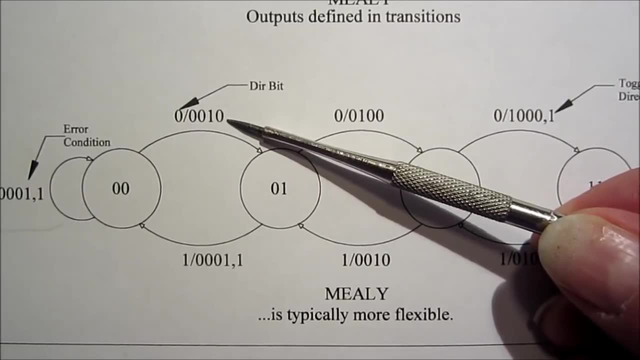 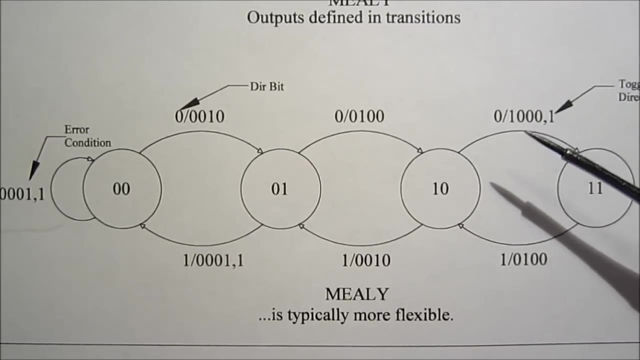 So in these states here we see our transitions, including an input which is the direction bit, but not outputting the direction bit. We're only outputting information that will power the output. Okay, So we're only putting out the LED output here. 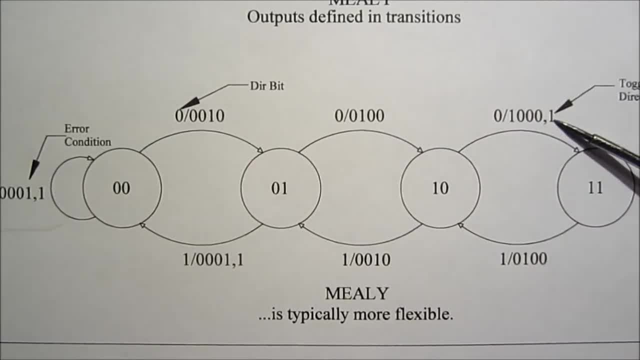 But down here, when we get to the end of the line, we do output a one to the toggle register and we toggle the bit. Now we're off in this direction again. we're only putting out, we're sensing or we're inputting. 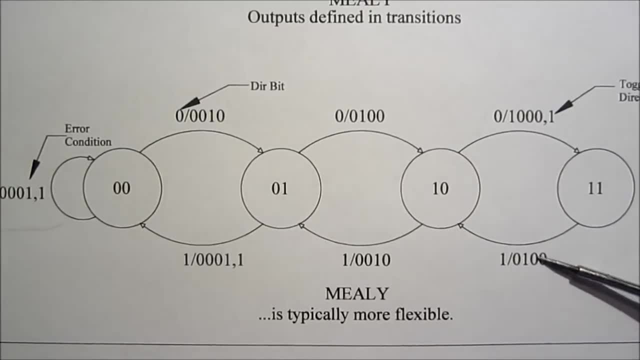 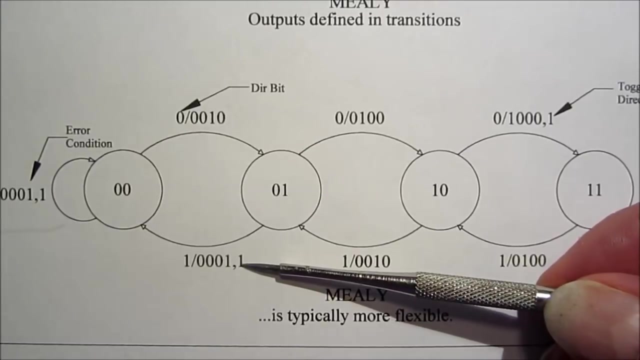 the direction bit and we're outputting LED information as we change states. And then we are sensing the input bit And we are outputting. We're outputting the LED information for the new state And then, when we get down here to the end of the line, we also output a toggle bit.